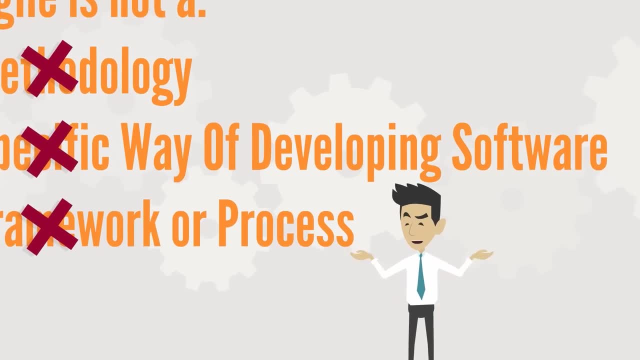 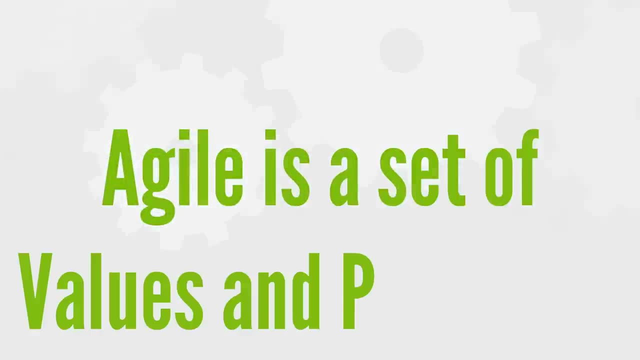 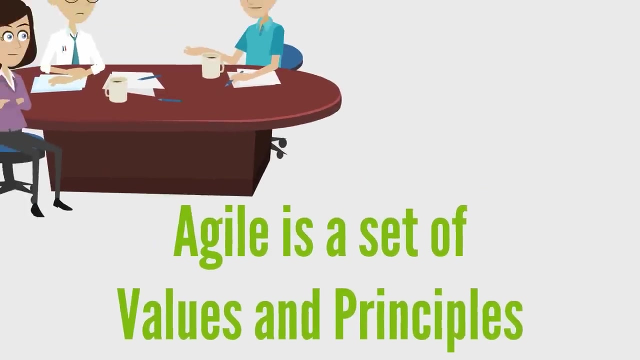 It isn't a framework or a process. In fact, most of the things that are marketed as Agile tend to miss the point of what Agile actually is. Agile is a set of values and principles. Much of the discussion around Agile has to do with following different practices, using 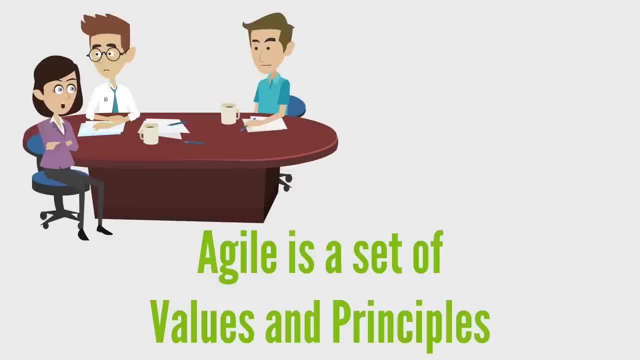 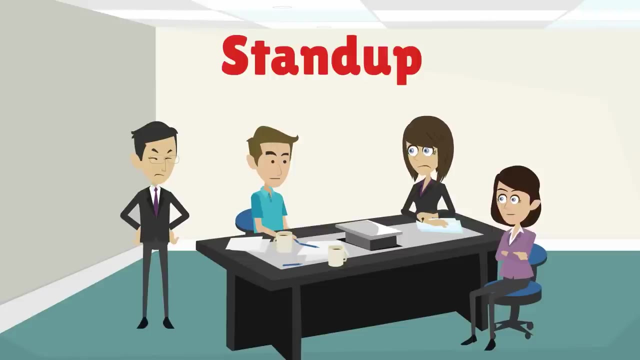 various methodologies and even developing with specific tools. While these things might help a team that's trying to follow Agile, they aren't Agile in and of themselves. For example, While a team may find that having a daily stand-up meeting is helpful, the stand-up 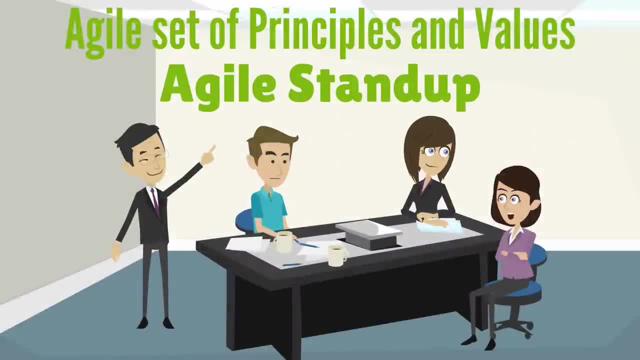 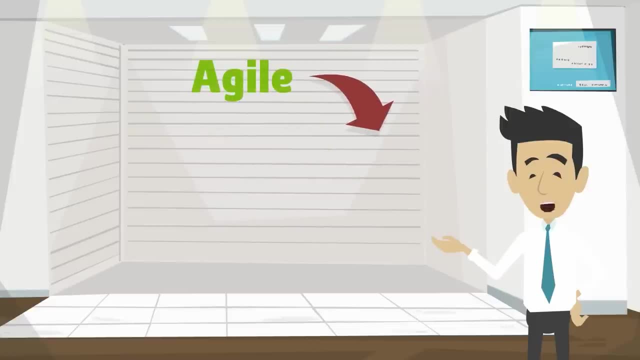 is only Agile to the extent that it is the result of a team following the Agile principles and values. When you understand this, it's easy to see that Agile is really a collection of beliefs that teams can use for making decisions about how to do the work of developing software. 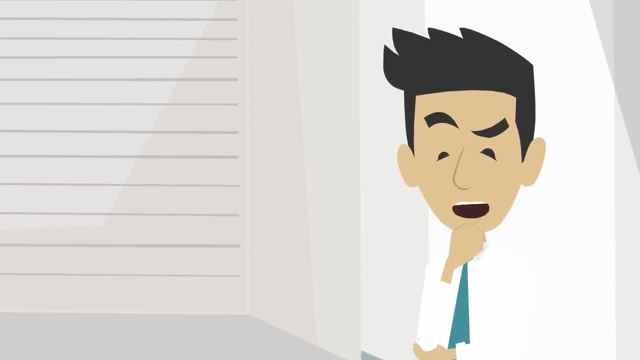 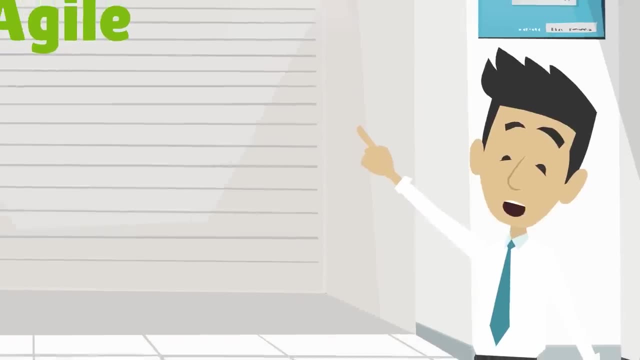 While this means the term Agile gets subjected to a great deal of abuse when people claim that this or that is the way to be Agile, it also means that if you truly understand what Agile is, it's surprisingly flexible. Agile doesn't make decisions for. 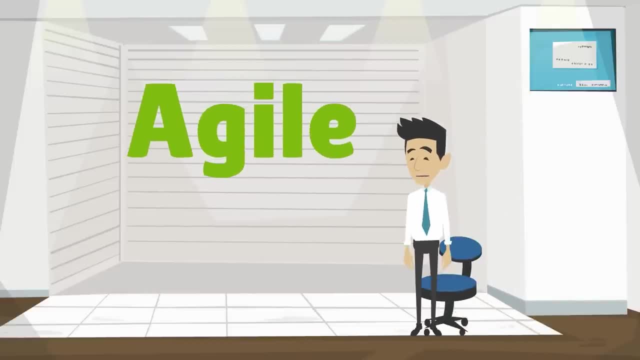 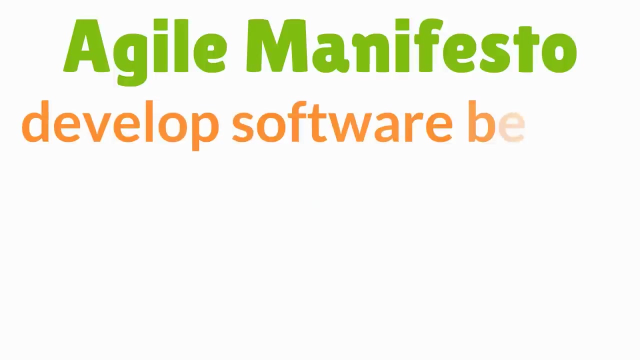 you. Instead, it gives you a foundation that teams can use to make decisions that result in better software development. The Agile Manifesto is only 68 words And it's very simple. It simply says that we can develop software better by valuing the items on the left side of the list more. 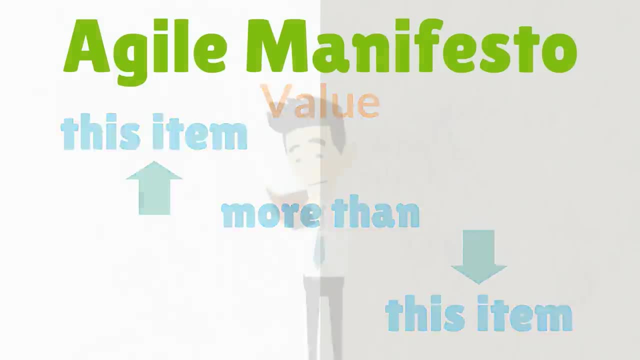 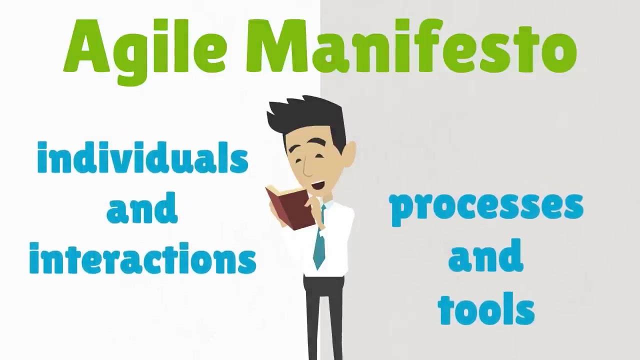 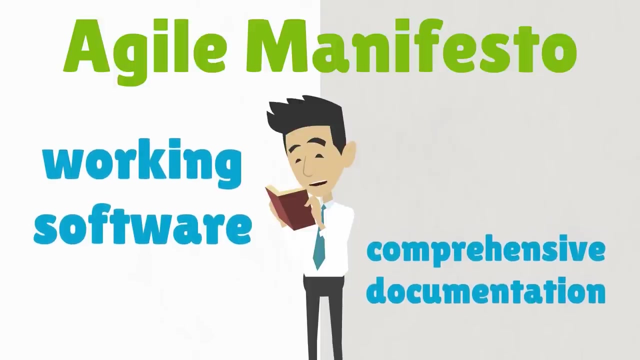 than the items on the right side. The Agile Manifesto says we are uncovering better ways of developing software by doing it and helping others do it. Through this work, we have come to value individuals and interactions over processes and tools. working software over comprehensive documentation. 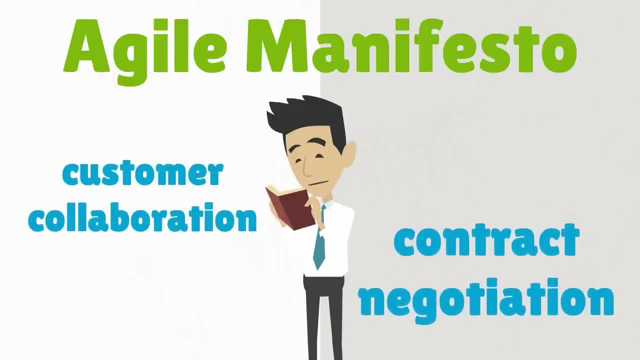 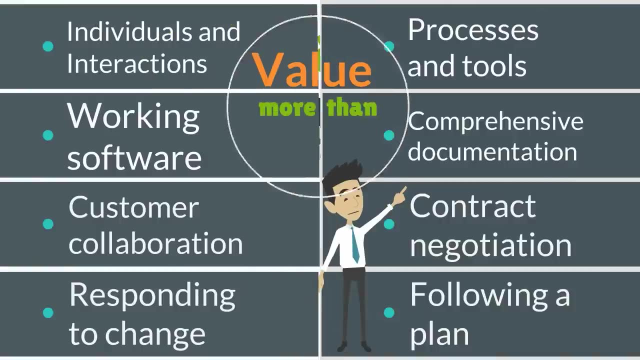 customer collaboration over contract negotiation, responding to change over following a plan. That is, while there is value in the items on the right, we value the items on the left more. In addition to the values of the Agile Manifesto. we value the values of the Agile Manifesto. 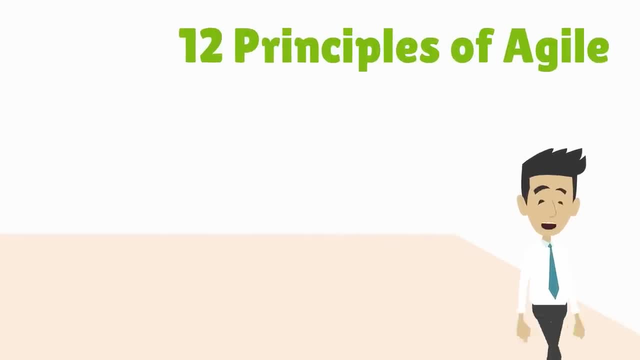 In addition to the values of the Agile Manifesto. we value the values of the Agile Manifesto. we value the values of the Agile Manifesto. There are 12 principles that support the values. Once again, the principles are very general and are less about telling you. 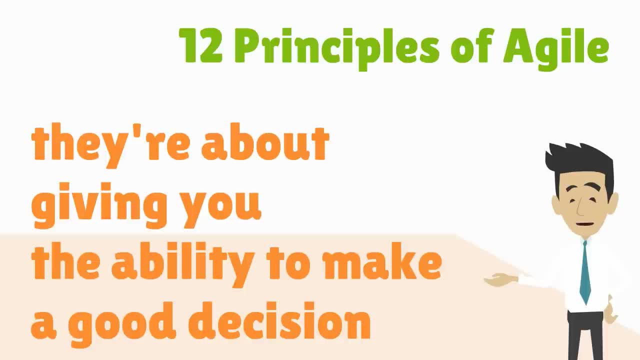 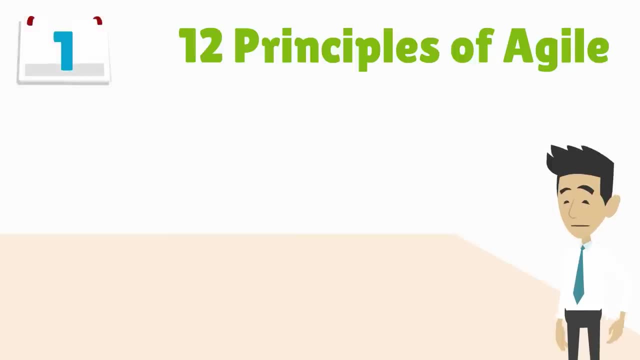 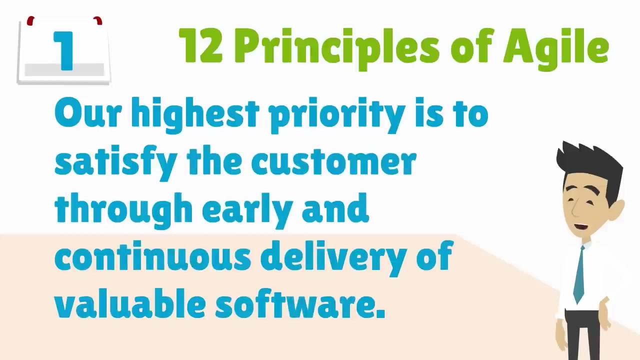 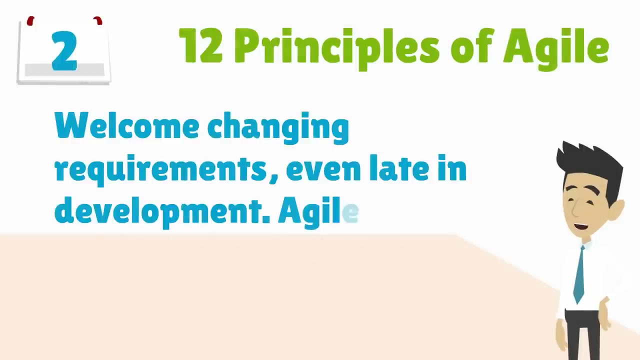 what to do, than they are about giving you the ability to make a good decision in a particular situation. The 12 principles are: number one: our highest priority is to satisfy the customer through early and continuous delivery of valuable software. Number two: welcome changing requirements even late in development. Agile processes harness. 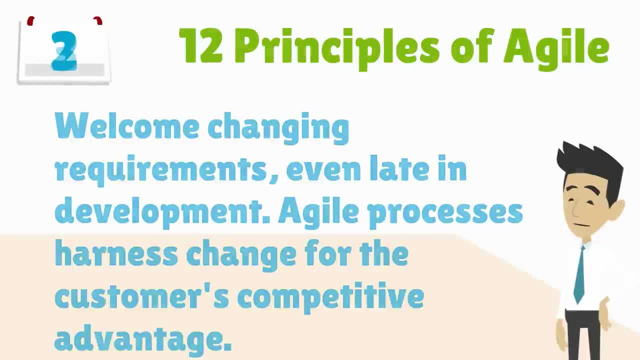 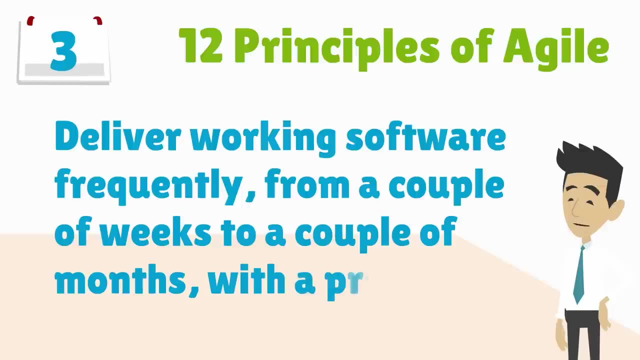 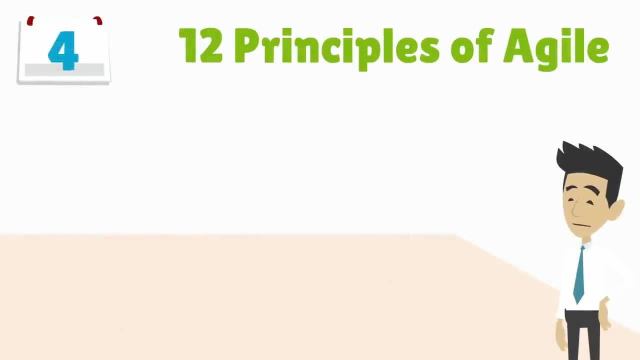 change for the customer's competitive advantage. Number three: deliver working software frequently from a couple of weeks to a couple of months, with a preference for the shorter timescale. Number four: business people and developers must work together daily throughout the project. Number five: build projects around motivated individuals. Give them the 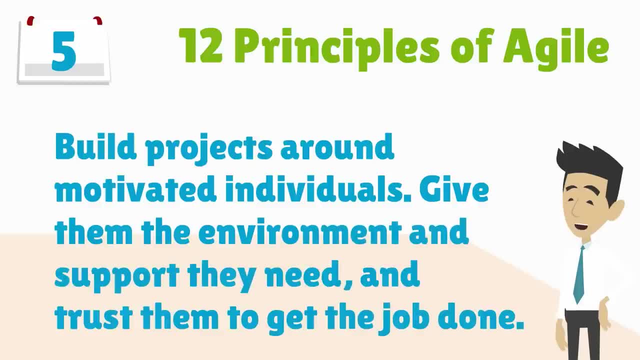 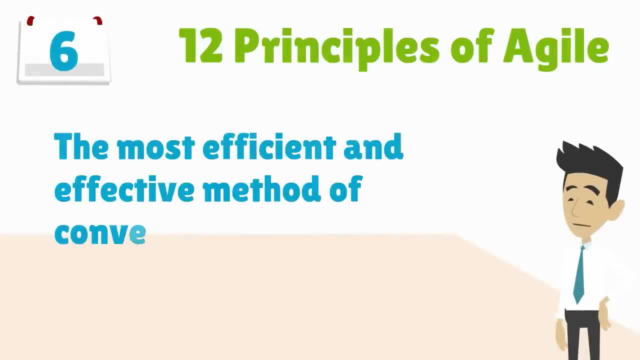 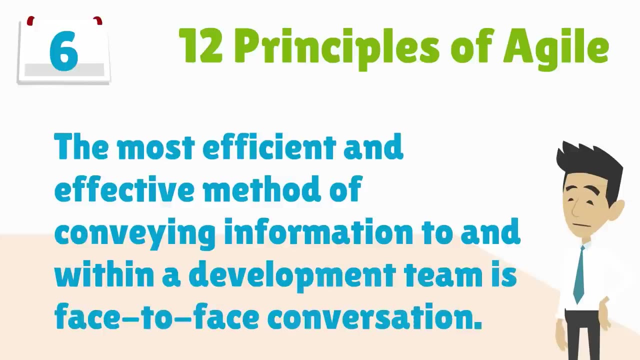 environment and support they need and trust them to get the job done. Number six: the most efficient and effective method of conveying information to and within a development team is face-to-face conversations. Number six: the most efficient and effective method of conveying information to and within a development team is face-to-face conversations. 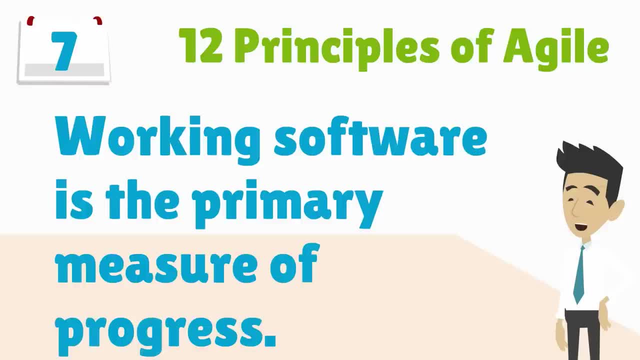 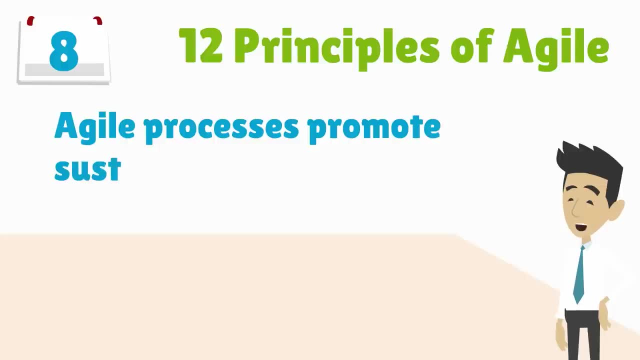 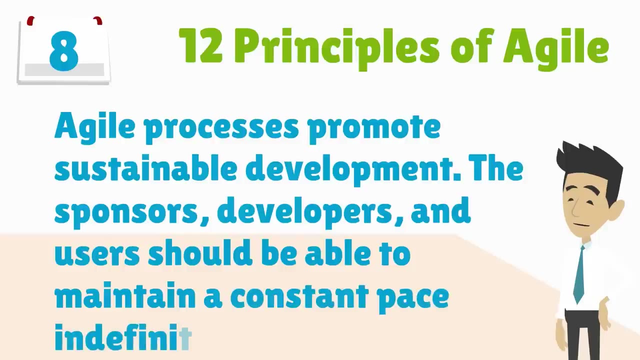 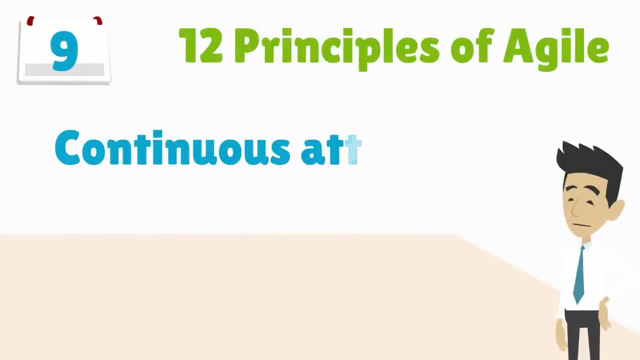 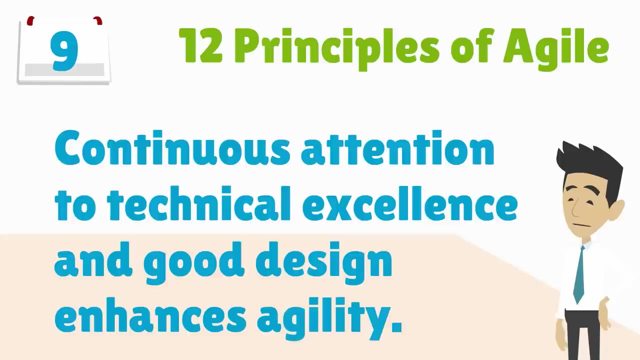 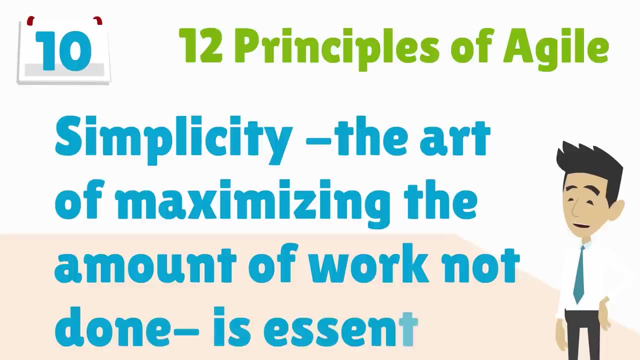 seven: working software is the primary measure of progress. Number eight: agile processes promote sustainable development. The sponsors, developers and users should be able to maintain a constant pace indefinitely. Number nine: continuous attention to technical excellence and good design enhances agility. Number ten: simplicity- the art of maximizing the amount of work not done. 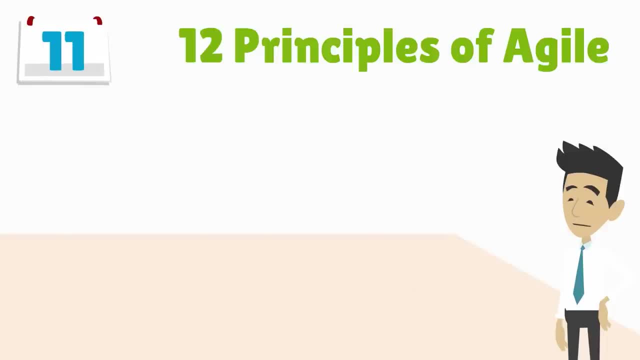 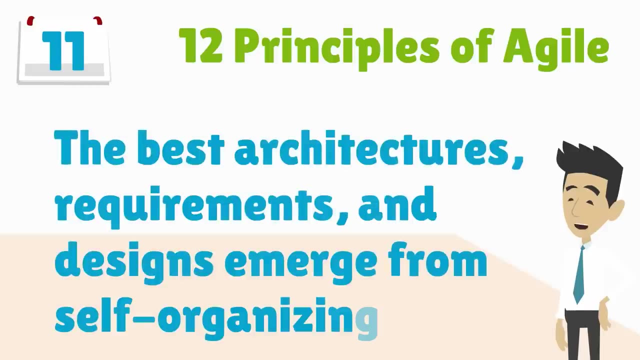 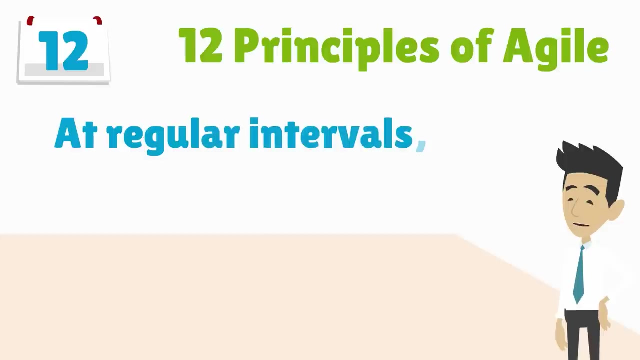 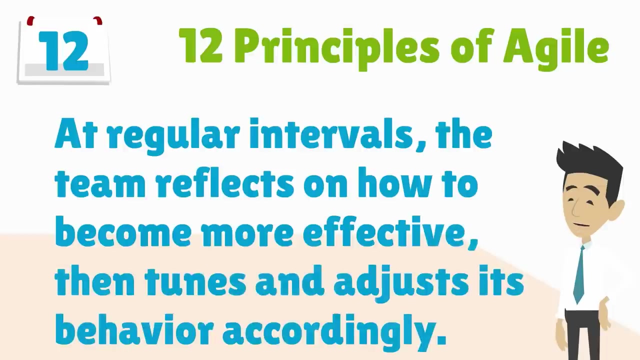 is essential. Number eleven: the best architectures, requirements and designs emerge from self-organizing teams. Number twelve: at regular intervals, the team reflects on how to become more effective, then tunes and adjusts its behavior accordingly, Since agile is a 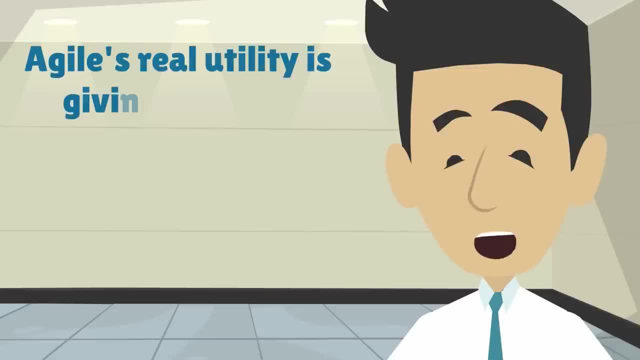 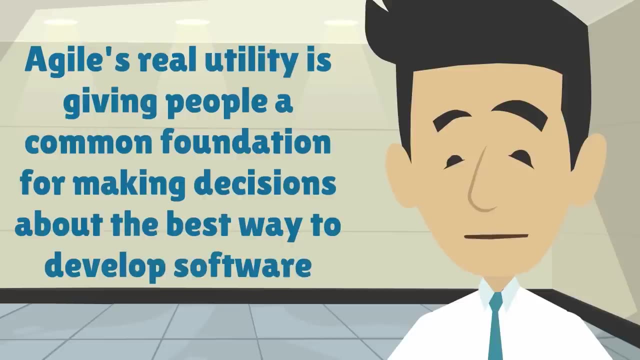 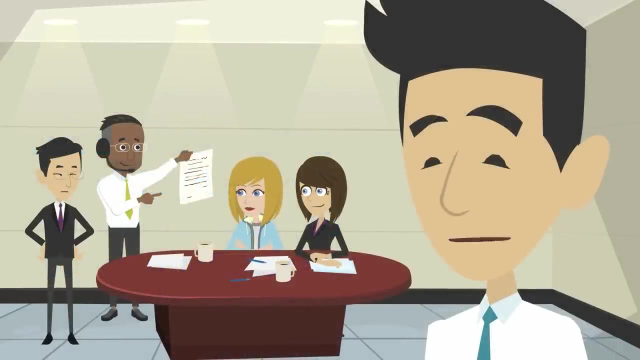 collection of values and principles. its real utility is in giving people a common foundation for making decisions about the best way to develop software. For example, consider a new project, A team that is in discussion on how to get requirements from the business owner. The suggested approach is to require that the business owner write. 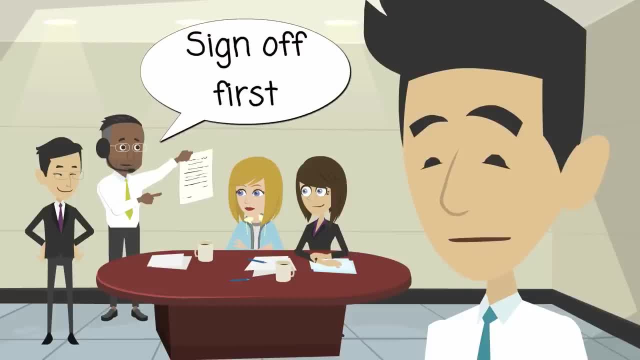 down all the requirements and sign off on them before beginning the work. A team that is following agile, would say. while that might work, isn't that inconsistent with our belief that we should value customer collaboration over contract negotiation, And doesn't it violate our principle that says the developer? 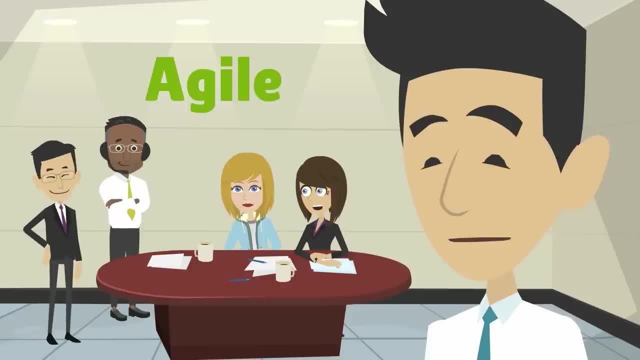 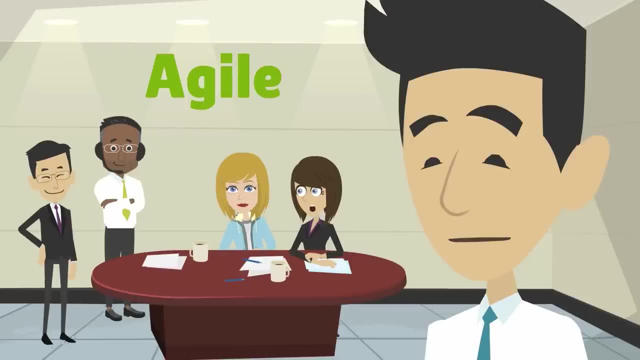 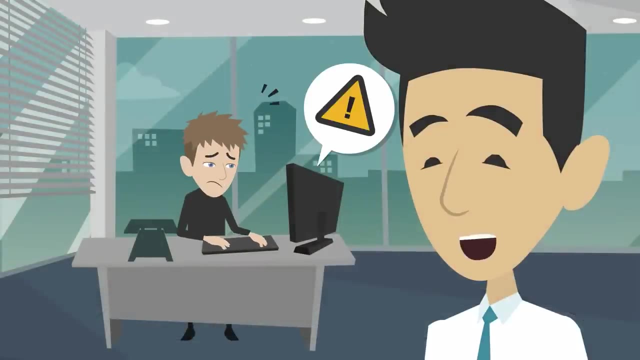 developers should be working with the business owners every day. How can we make this decision in a way that is consistent with our values and the principles we follow? Or consider a developer who's working on implementing a feature for the business owner. The developer realizes he needs a database to make the feature work. 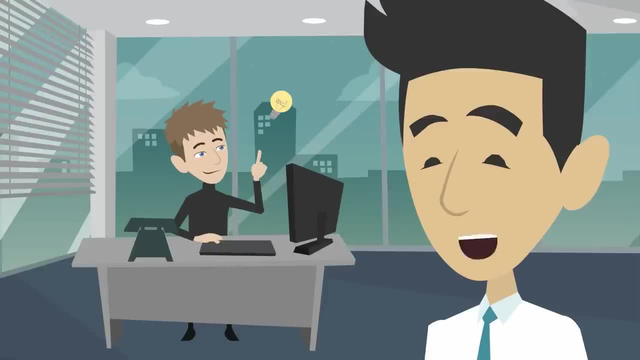 The first idea that comes to mind is to stop work on the feature and build out a robust database layer that will handle the needs of the feature and provide support for other development that will be needed later, If the developer believes in the Agile values and is trying to follow the Agile principles. 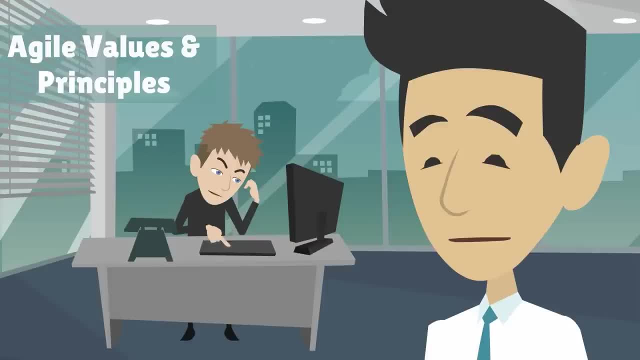 they would think. but building out this layer means I would have to delay delivering what the customer can see as valuable software they can use. If I can find a way to build just what is necessary to deliver this feature, it will better align with my purpose. 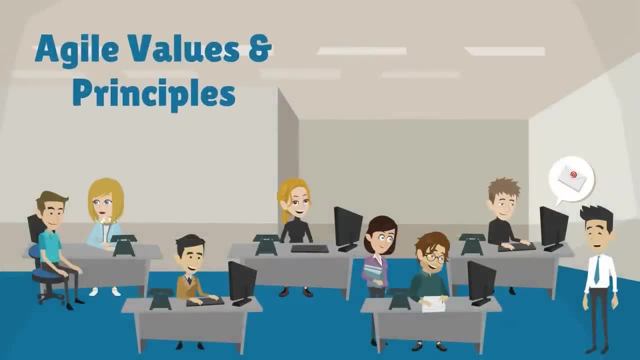 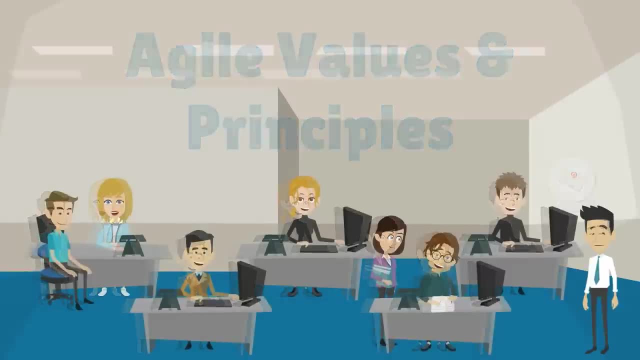 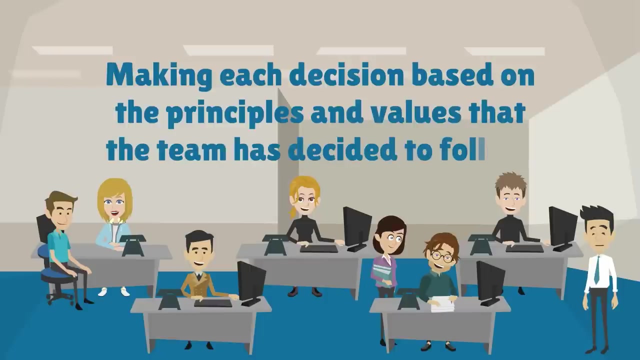 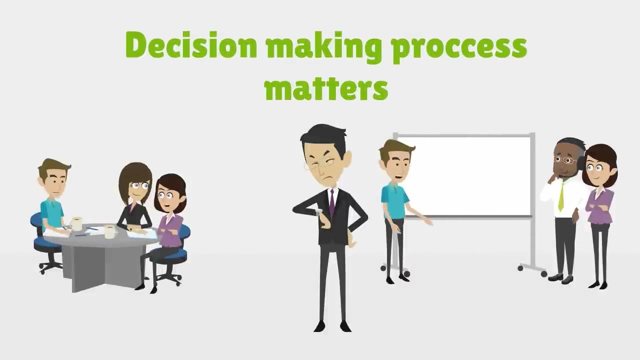 When you have a team that is following Agile, they will be making hundreds of decisions each week in the way described. That is what it means to be Agile: making each decision based on the principles and values that the team has decided to follow. The decision-making process matters. 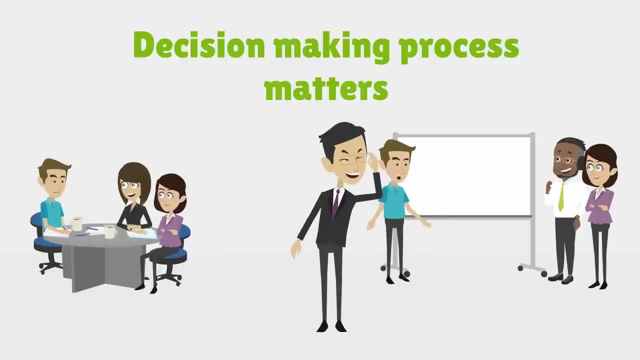 You can't try to short-circuit things By taking decisions Made by another team And just blindly doing what they decided to do. Another team may make decisions based on the Agile principles and values that end up with a particular way of doing their work. 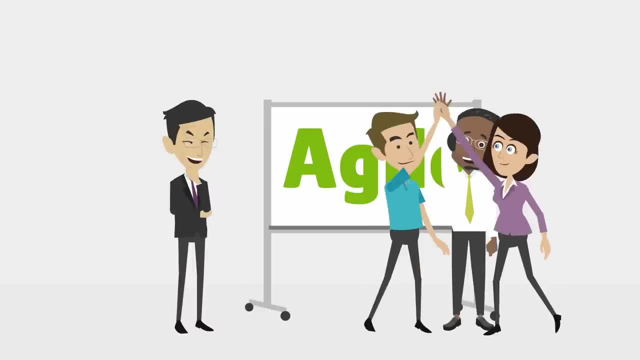 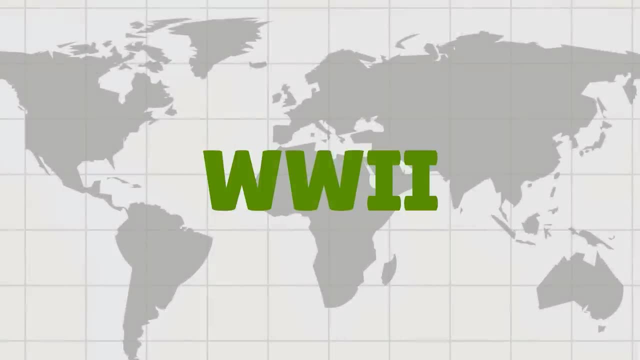 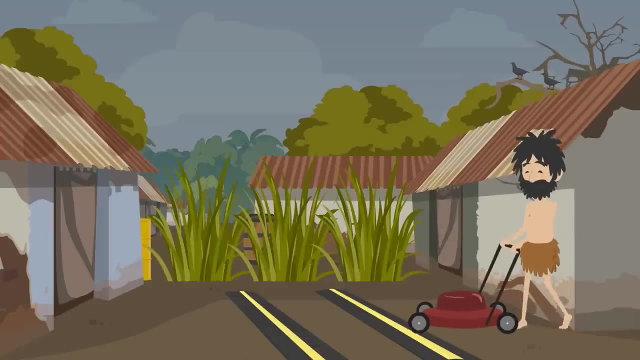 Simply trying to mimic another team's actions and practices won't make your team Agile. After World War II, Melanesian islanders were observed trying to bring cargo planes and their supplies from the sky by mimicking the practices they had seen performed during the war. 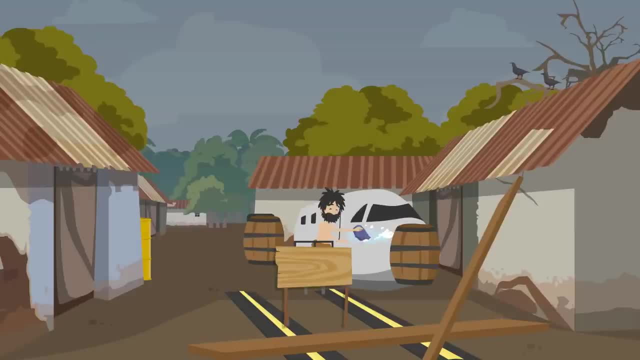 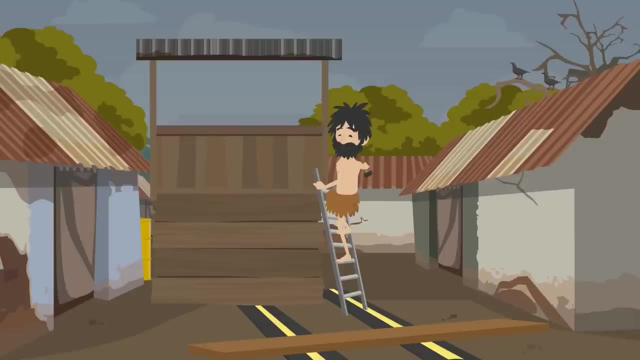 This included clearing the forest to make a landing strip complete with full-sized planes made out of straw. They also created structures that mimicked a control tower out of bamboo and had someone sit in it wearing headphones fashioned from coconuts. It's easy to fall into similar type of cargo cult mentality when it comes to making cargo. 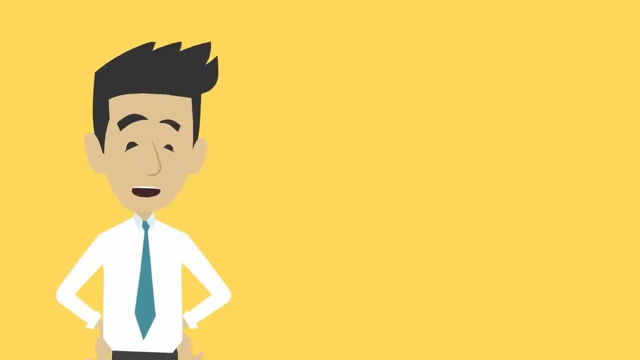 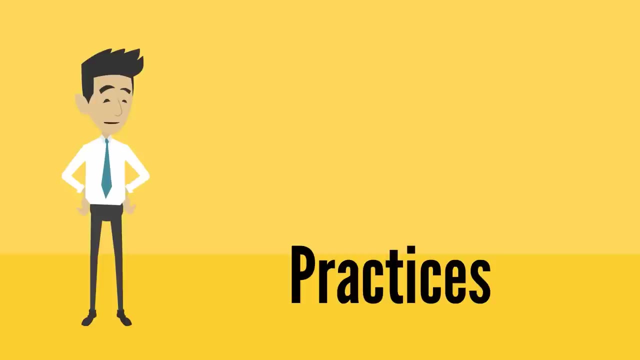 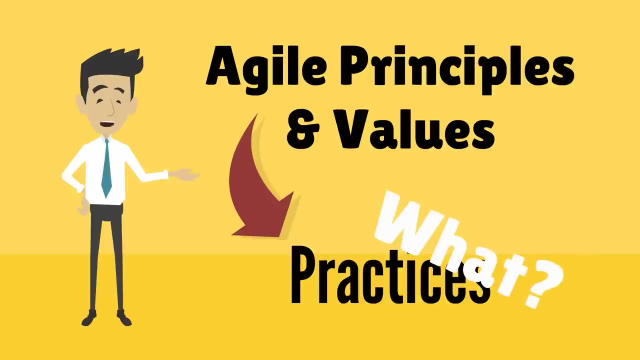 planes. But when it comes to Agile, the things that are easy to notice in a highly functional Agile team are the practices they are using. But the practices a team uses are the result of following Agile principles and values. It's less important what practices a team happens to be using than why they are using. 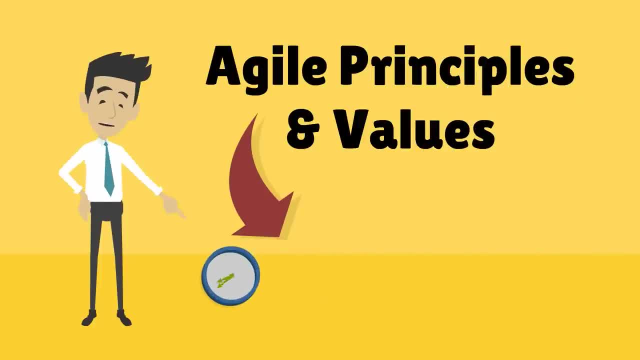 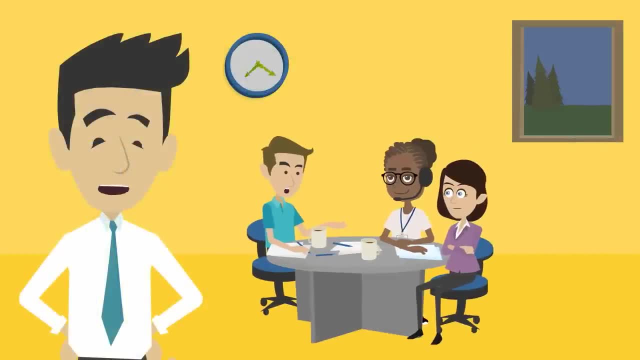 it. In fact, as time goes by, a good Agile team is probably going to change and refine their practices that they use. A team might start with Scrum and later find that Kanban is a better fit for delivering value to their customers. 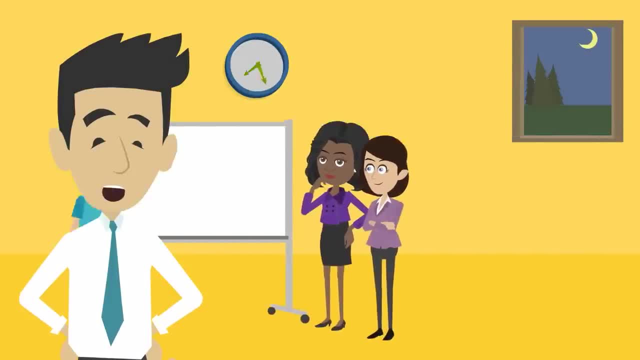 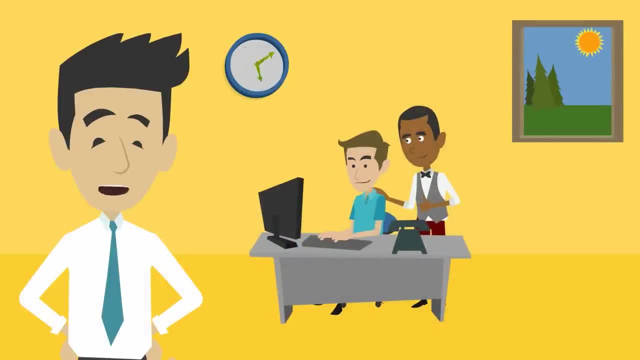 A team might begin standing up on daily meetings and later decide it works better for everyone to stay sitting down. Another team might start out using planning poker to estimate story size and later do away with story points and simply split stories to be approximately the same size. 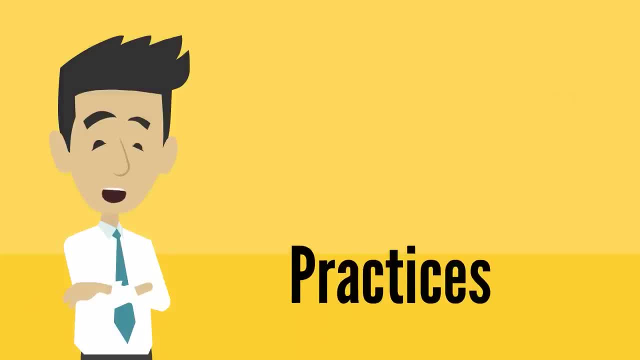 That isn't to say it's useless. It's just a matter of time before you start using it. It's just a matter of time before you start using it. It's useless to look at practices being used by teams that are performing well. 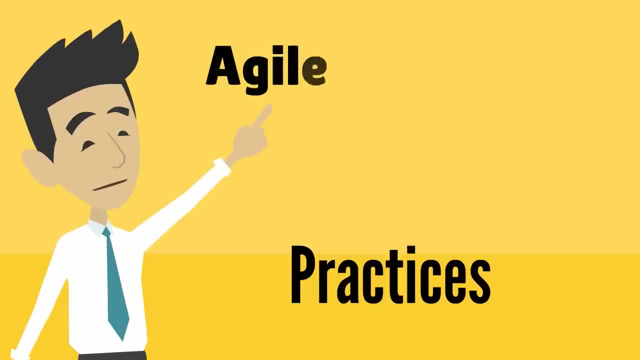 But you can't go looking for practices to make you Agile. Your principles and values are what will make you Agile. You have to look for practices that support your principles and values. The way you select your practices is what determines whether you are being Agile or